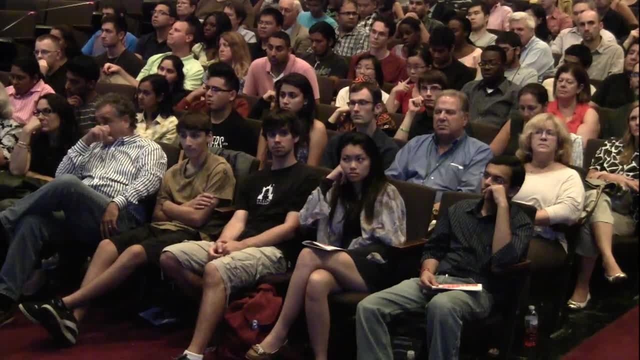 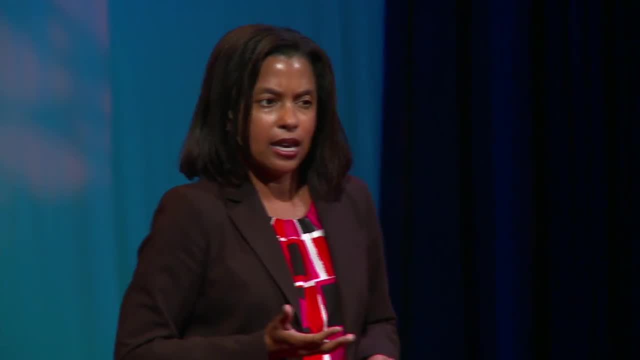 put them back. So how do you decide? So stem cells have been the popular cells, What we're cells of choice because of that. So stem cells can virtually turn into any cell type in the body, And so we've been focusing on adult cells, adult stem cells. Why is that? Because virtually every 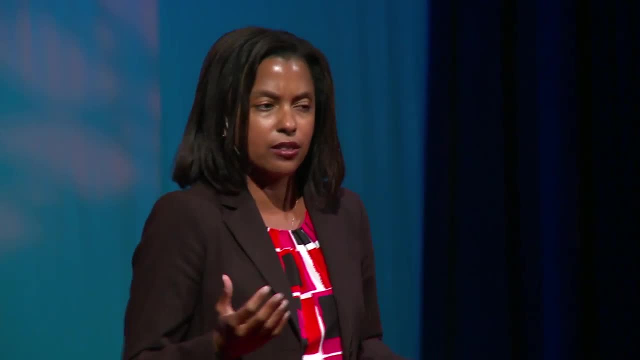 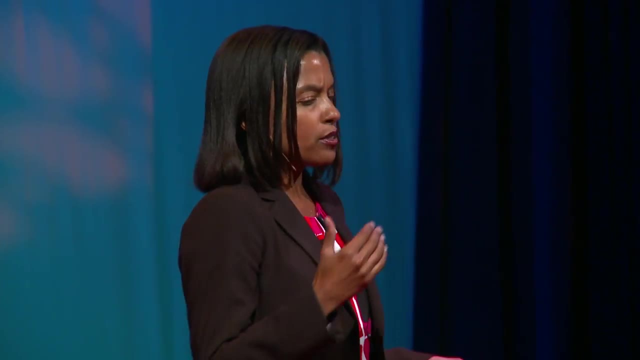 tissue in your body contains a very small reservoir of these cells, of these stem cells. If you can isolate them, you can grow them up pretty easily in the laboratory. So we've been focusing on bone marrow, these bone marrow stem cells, And those stem cells have been well 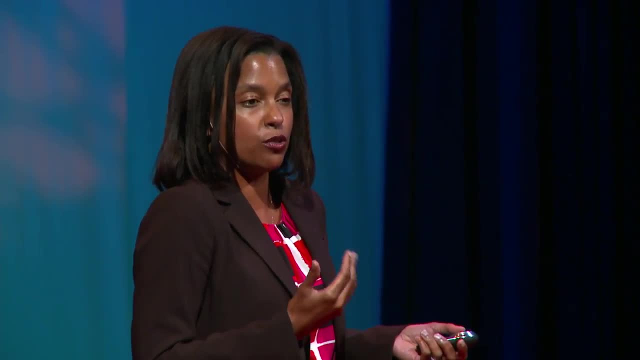 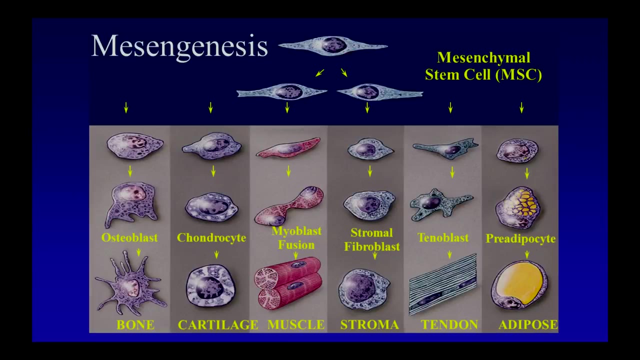 characterized over the past- really 20,, maybe 30 years- have been used clinically, have been proven to be safe and can actually repair tissue. So we specifically use these mesenchymal stem cells. And why do we use them? Because we're interested in repairing orthopedic tissue, the bone and the 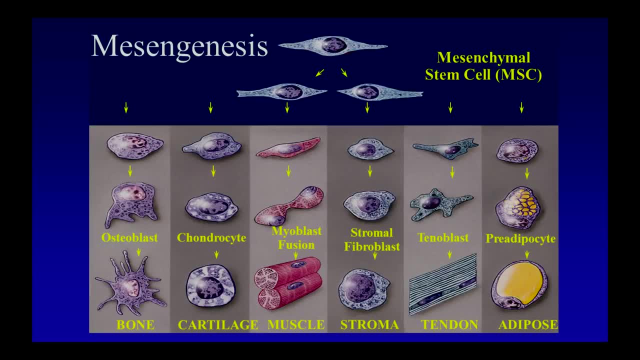 cartilage. So those stem cells can really turn into all these different cell types that are shown here. but we need to provide the right cues that they kind of stay on track and turn into those cells that we want them to go to turn into. So bone marrow stem cells. 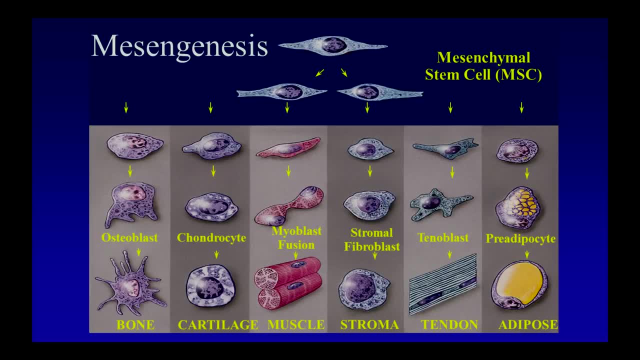 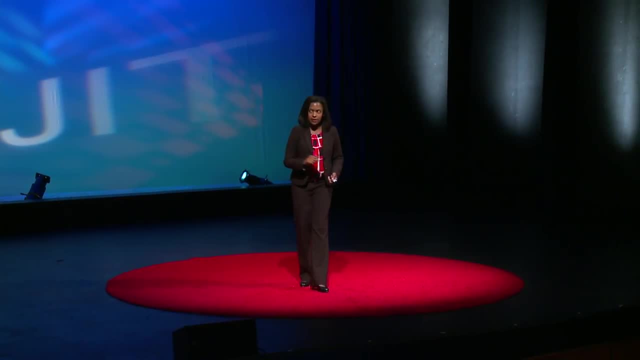 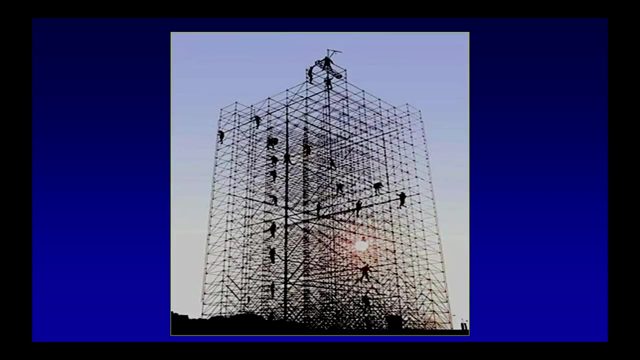 Bone and cartilage. So how do we do that? All those little steps, those arrows, you've got to provide those right cues, And so that scaffold is the key. So you can think of a scaffold analogy where that scaffold is sitting up inside a large building, So workers get on that scaffold. 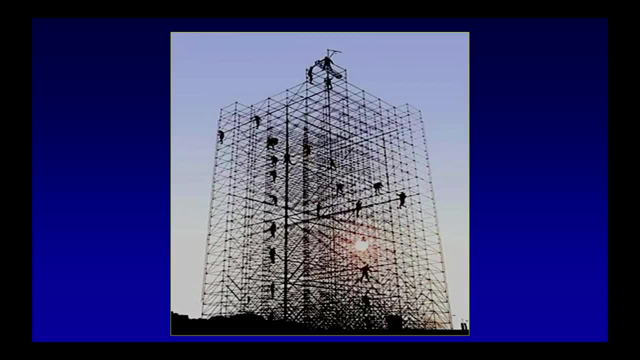 it supports them, helps them repair the building. So the cells, the small scale, that's essentially what our scaffold, our biomaterial, is doing. in the body, The cells jump on, attach needs to support their attachment and support their ability to synthesize this tissue. 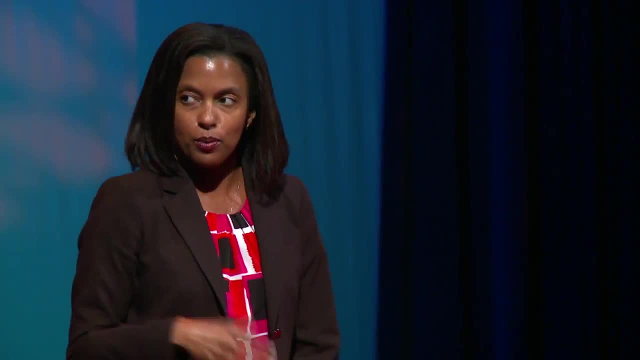 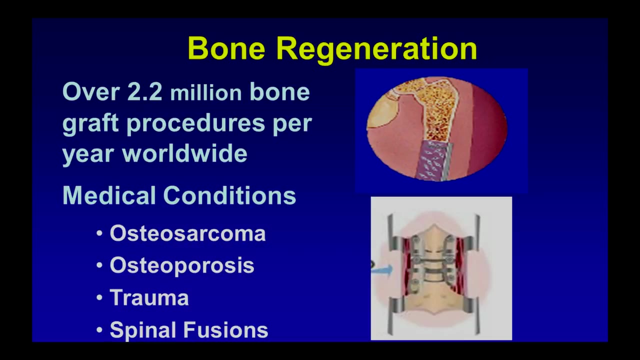 make this tissue. So what about these problems, these big problems? So bone repair We're talking about here. there's over 2.2 million bone graft procedures okay, worldwide per year, And so these are used to treat these very large defects that will not repair okay themselves, And so 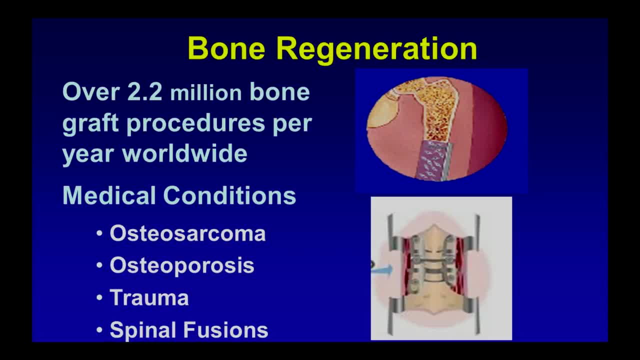 bone grafts have a very limited supply. You have a very limited amount of bone They can actually be used for yourself And donor bone from people or even cadavers are very limited in terms of their ability to even work. So we use these strategies, the stem cell strategies, to 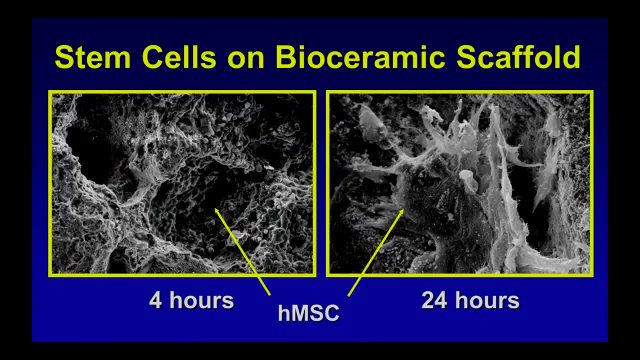 repair these very challenging defects, And so we've developed this scaffold here. It's porous, so it's got these large pores Cells actually sit on it, And it also has these very small little features, kind of granular features in the scaffold that help those cells to attach The 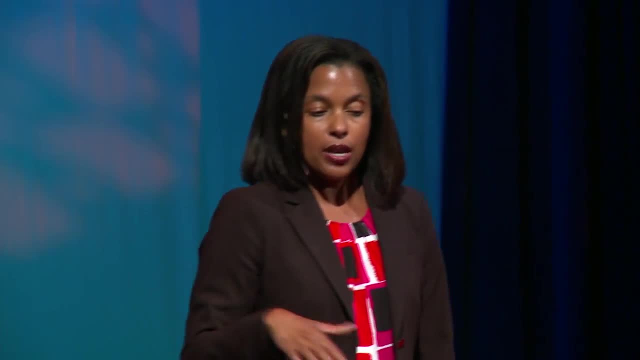 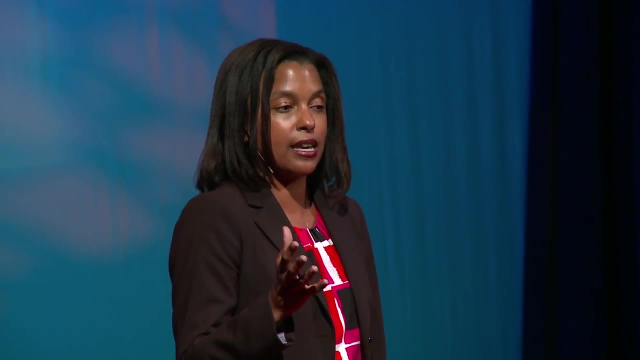 cells actually ankle and they can actually attach to each other. So it's a very large themselves down on those features and so we made that architectural design. but also it's composed of a bio ceramic, so that ceramic contains calcium and phosphorus, so that specific chemistry stimulates those cells to actually turn. 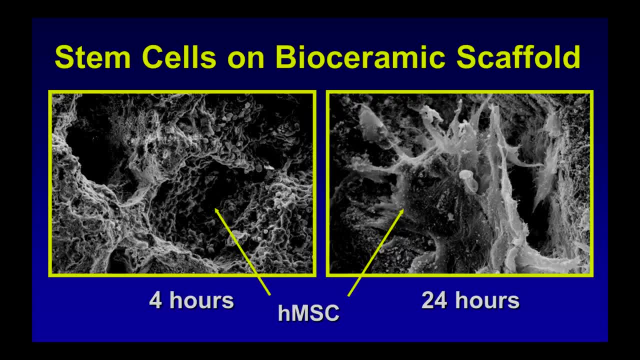 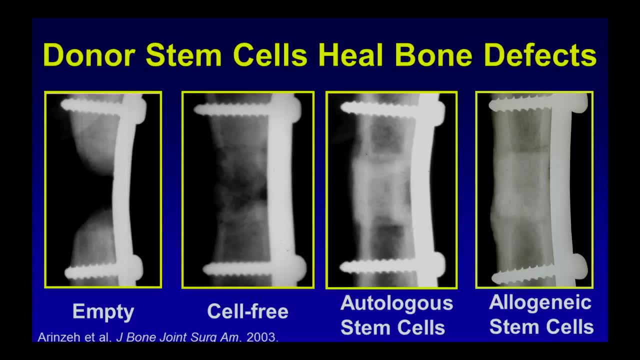 in turn into bone cells. calcium phosphate is normally in your bone tissue, so we're using that as the chemistry for the scaffold to get the cells to turn over and form bone and they form a lot of bone. so here we have a defect there on the far, on the far left, and that defect in the bone. 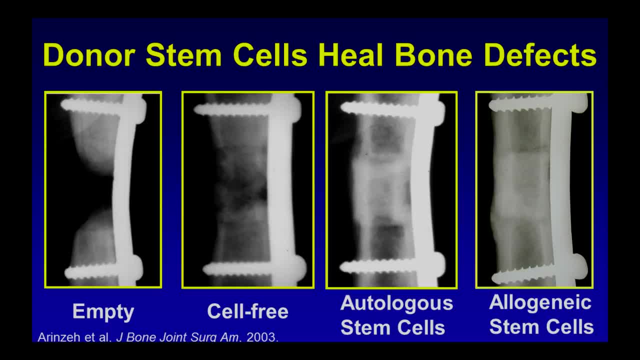 normally will not repair itself. but if you treat it with the stem cells on that scaffold it will fill in with with bone okay over a period of time and completely heal that defect. and so what we've discovered is one that scaffold works to drive the cells, but also the stem cells can come from that patient. 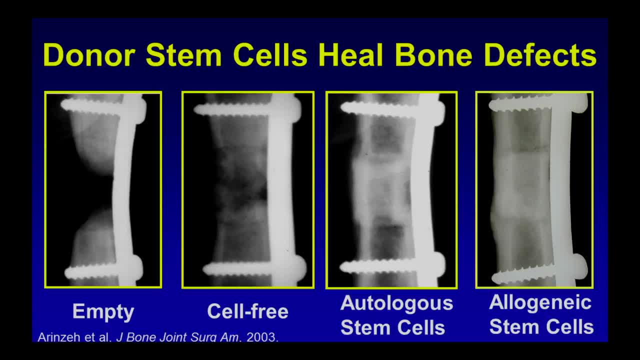 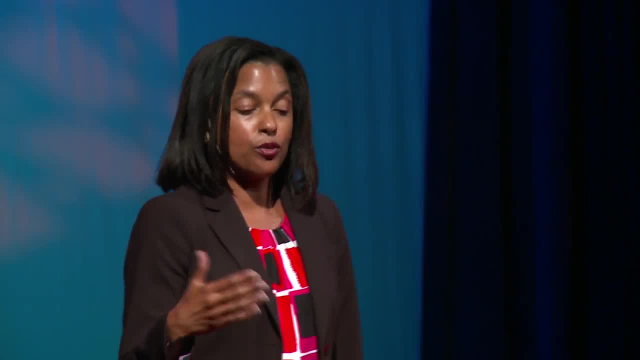 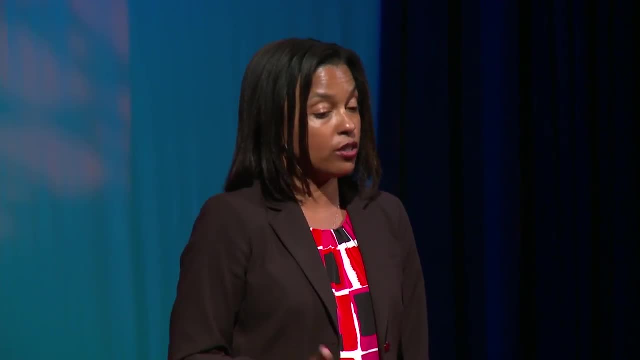 him or herself, but they also. we can get them from donor. they can be donated stem cells from a, from a person that's completely unrelated from that patient. so we can use donor, or what we call allogeneic stem cells in that tissue and it will fully repair that tissue and will not cause rejection, and so that's a. 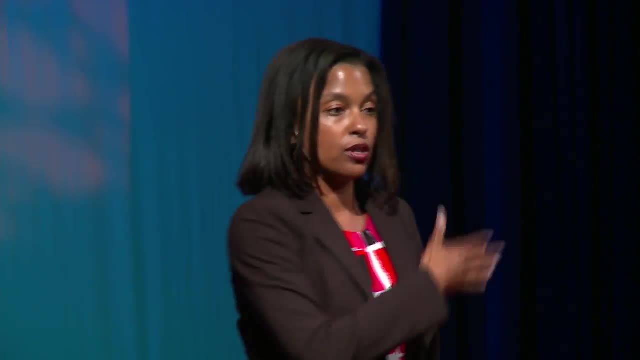 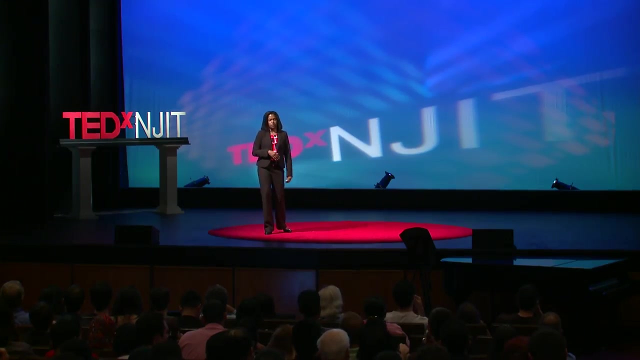 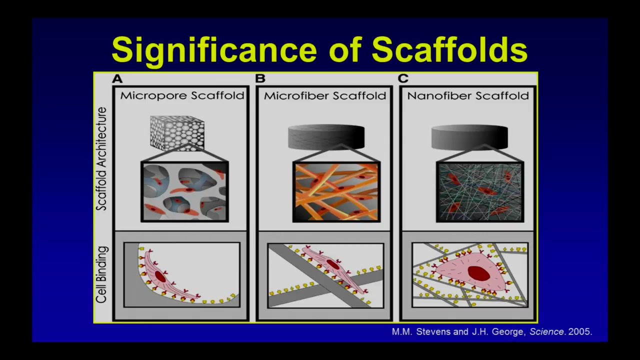 major finding because those cells can be used and you don't have to use immunosuppressive therapy on on these patients. they can heal and heal very readily. so we can improve upon that discovery. okay, that's actually now a product osteocell that's in use. We can improve upon that bone formation or rate of bone. 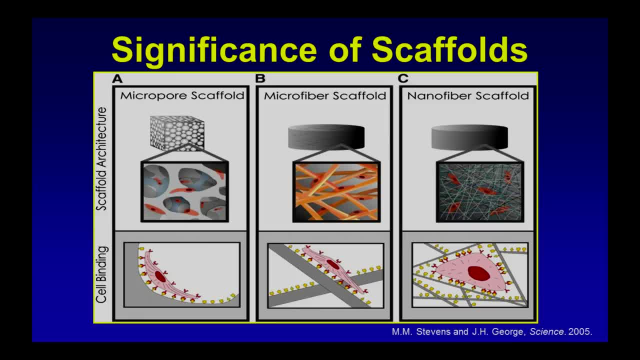 formation by the design of that scaffold, And so what I showed you before then was a porous scaffold that looks kind of like a sponge. So again, on that far left that you see there looks like a sponge, Fairly large pores in comparison to this. 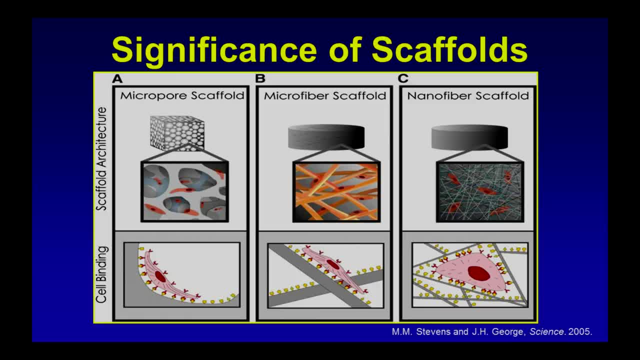 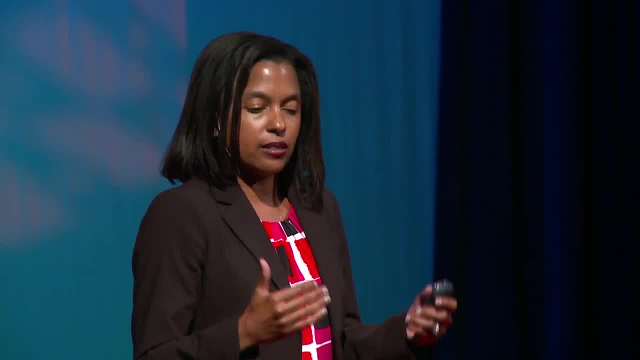 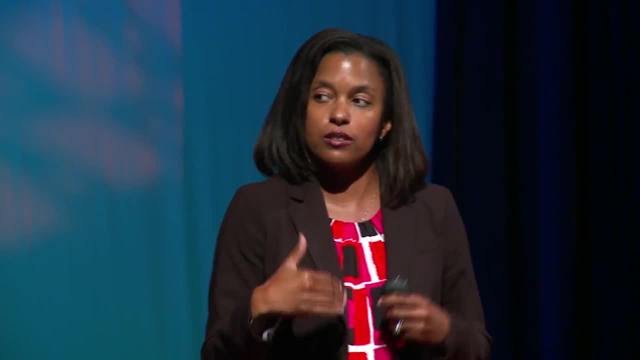 to the cell. So what the cell is actually sensing is more like a two-dimensional structure. But if you make features at a smaller scale so into these fibers, then the cells are actually sensing a little more of a greater surface area. So they're able to actually attach more readily to that surface because there's 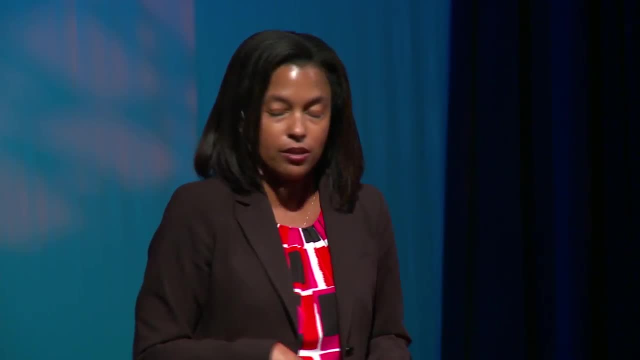 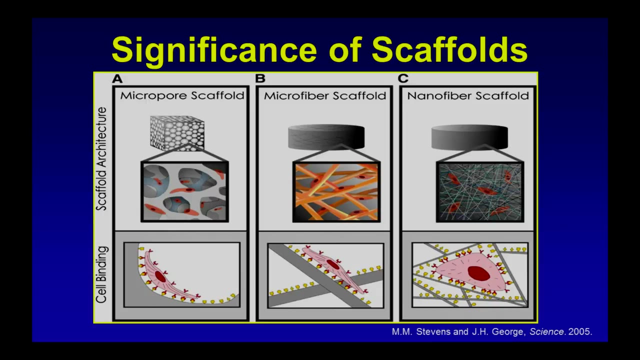 actually more, more area there for the cells to actually anchor themselves onto. Cells have little feet, You can think about it. they're called receptors, So they're actually attaching to proteins and proteins are sitting down onto your scaffold, So more of that protein interaction can happen with those cells. 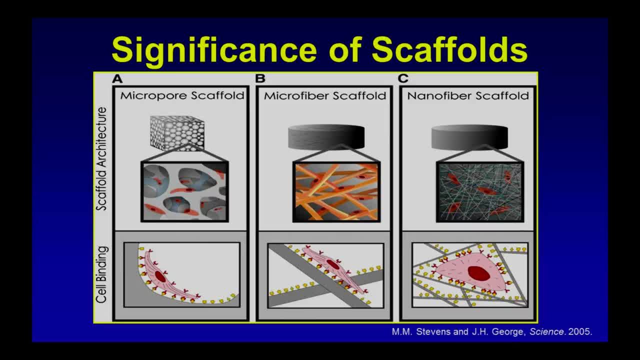 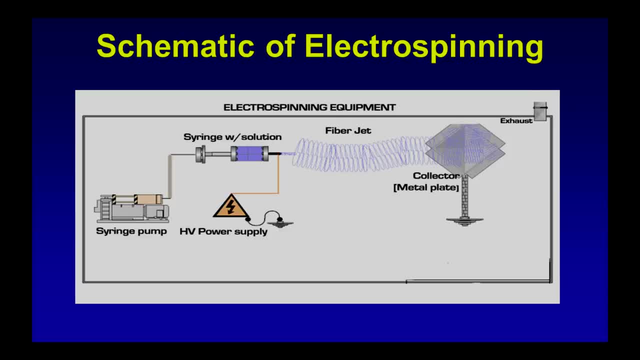 And then you can see that the cells are actually more easily attached to the protein. So if you get down even to the nanoscale, there's a lot of interaction, So cells attach really well. So we make these structures then using a process. 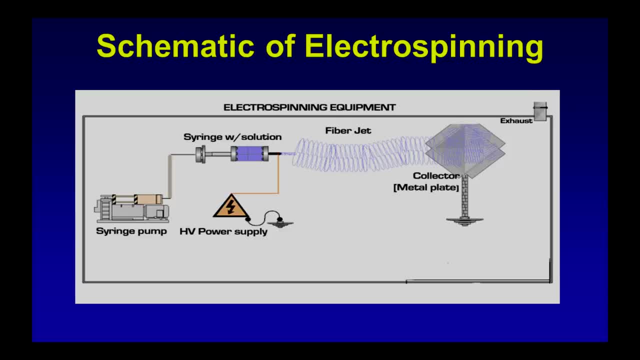 called electrospinning, And this electrospinning was actually developed in the textile industry. So it's like you know the the way you make clothing. okay, It's like the clothes that you have on. These are the scaffolding structures. 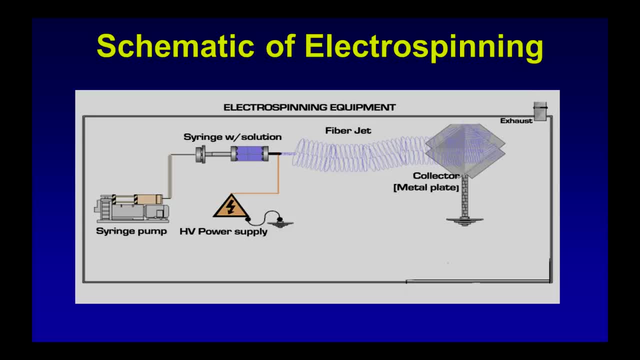 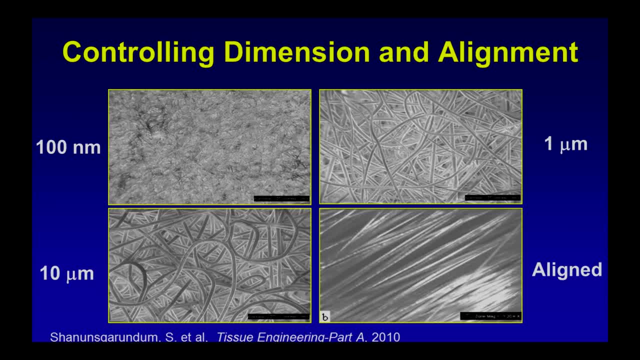 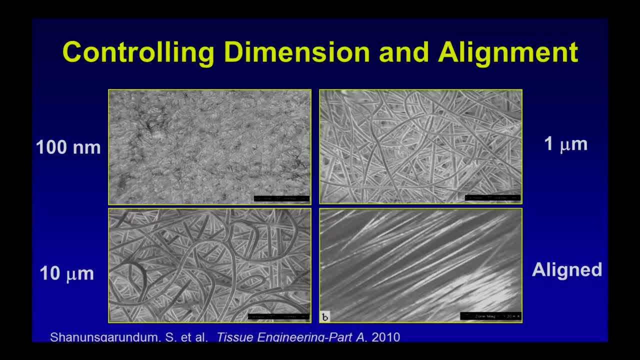 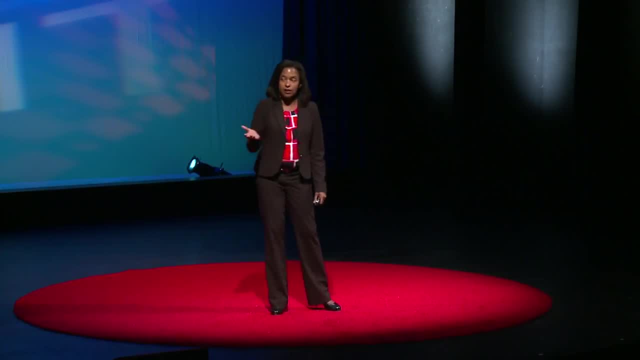 sized fiber structures and very large micron sized fibers, And we can arrange these fibers. You can be unorganized, what we call random, or we can make them aligned. Aligned is what you're seeing there in that lower quadrant, And so all. 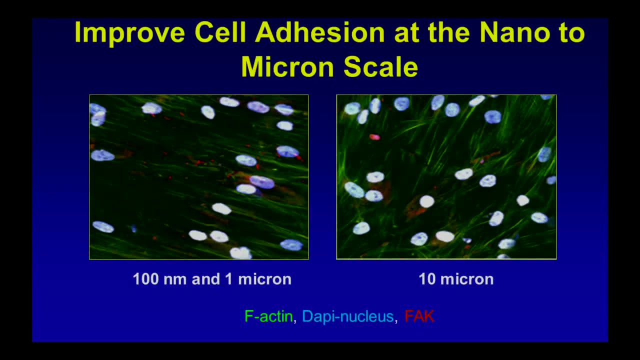 that's important again for cuing the cells. What we've been able to show is that nanostructure, and as you get to the lower, smaller micron size, does affect the way the cells really attach to the substrate. It improves attachment. 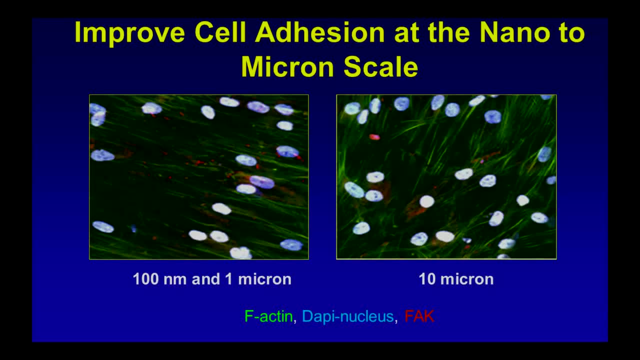 The cells here are the cell body. The cell body is staying there in green. You see how very organized it is. on the nanostructure, If you go up to higher, much larger micron fiber structures, the cells start to look a little unorganized. 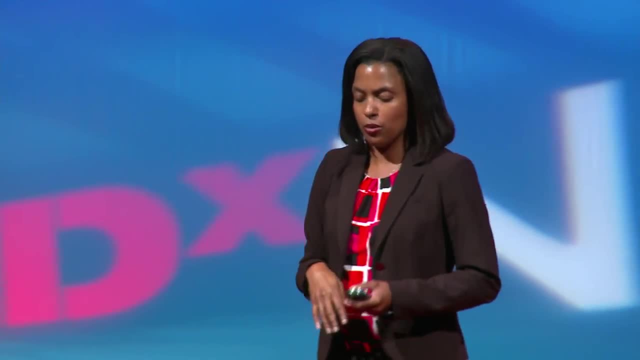 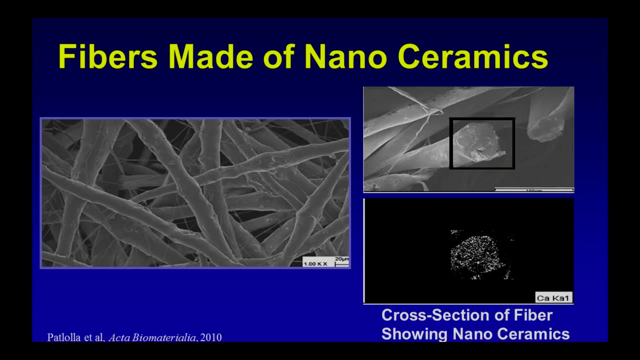 That green array actually looks fairly unorganized. So we improve attachment that way. So if we go back to that bone application, how do we actually improve the rate of bone repair? We've designed those materials. We're now using these fibers. We also incorporate one more interesting feature: We now use nanoceramics in those fibers. 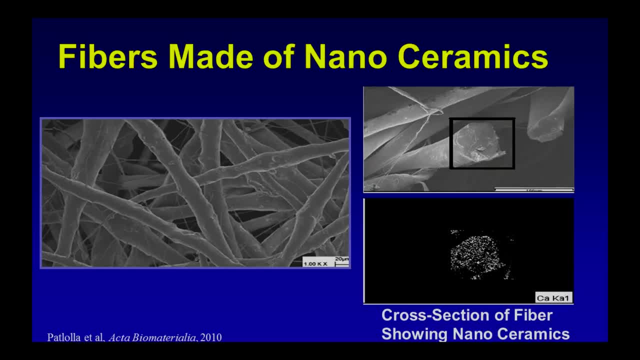 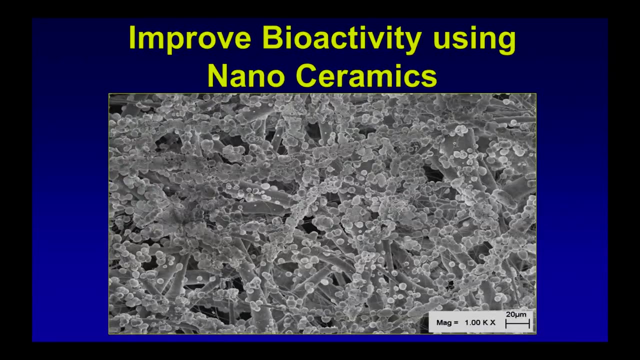 And those nanoceramics that are shown here are embedded and dispersed throughout the fiber, And so when you get down to this really small scale, those ceramics actually become extremely reactive. And so when you put that into the body, they become so reactive that they actually form what's called bone. 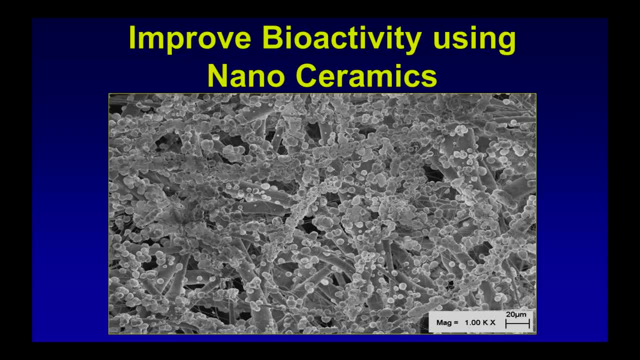 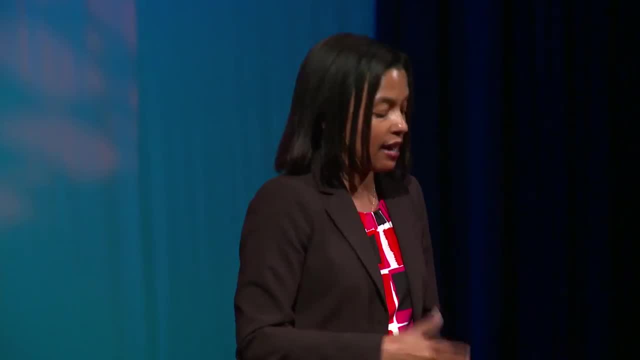 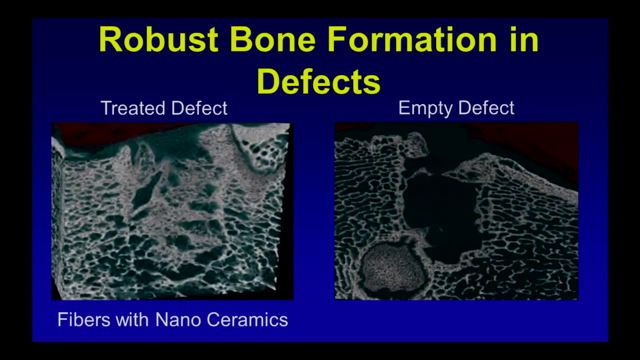 Bone mineral on the surface of these materials And that's really important again for the cells to actually begin to form bone tissue, So that reactivity we've been able to show in these bone defects, Just the material alone will rapidly produce, quickly produce new bone tissue. 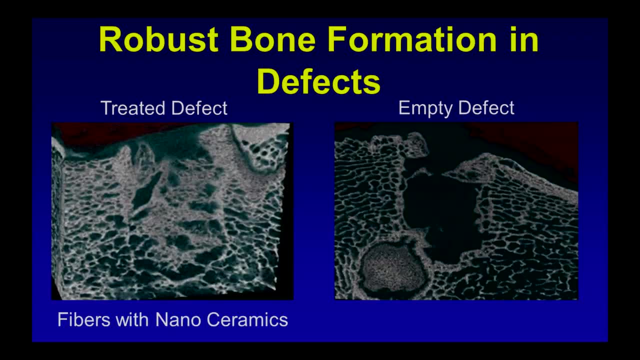 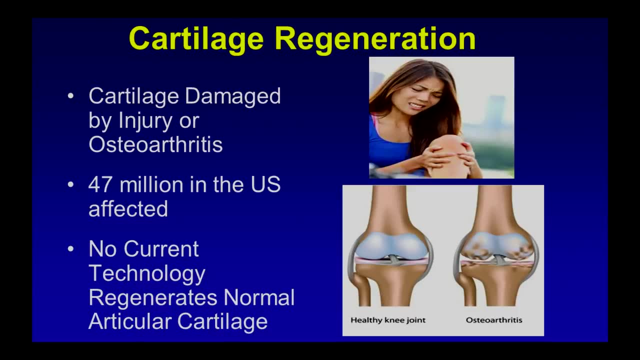 So it fills in very quickly because those nanoceramics start to react so quickly. An even more challenging medical problem is cartilage or the repair of cartilage. So if you get injured due to a sports injury or maybe just long term as you age, as you become older, 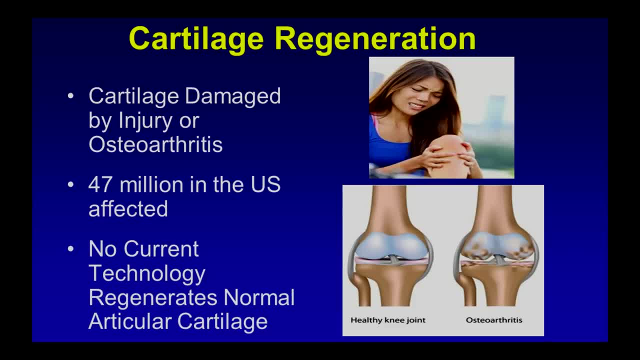 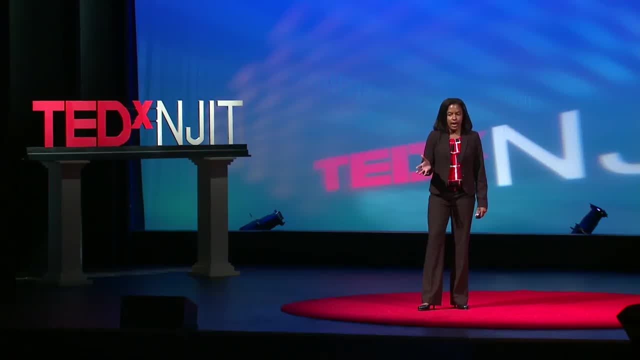 you start to tear and tear there in your cartilage. Cartilage will not repair itself. And so, yes, okay, Cartilage will not repair itself. And so and it becomes damaged. it can become so severely damaged that it will lead to osteoarthritis. 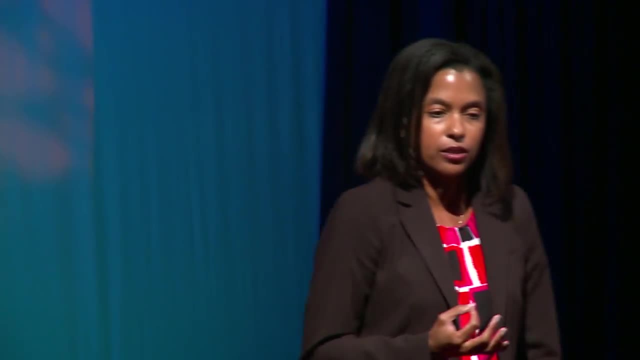 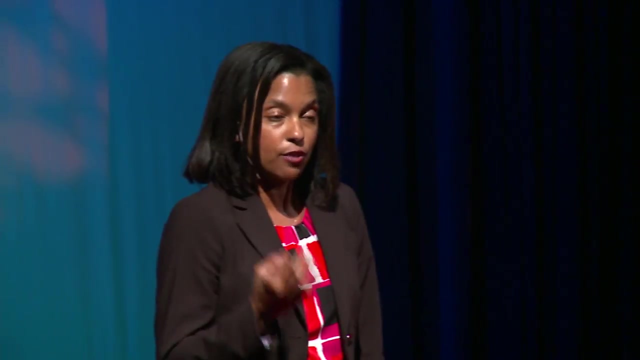 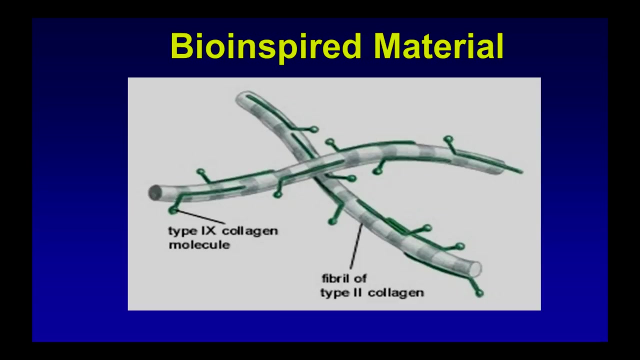 So over 40,, so 47 million Americans suffer from this condition. So there's currently no technology out there that will repair this normal cartilage to the point where it's actually functional again. So we've taken a bio-inspired approach And similar to what really I've been talking about. 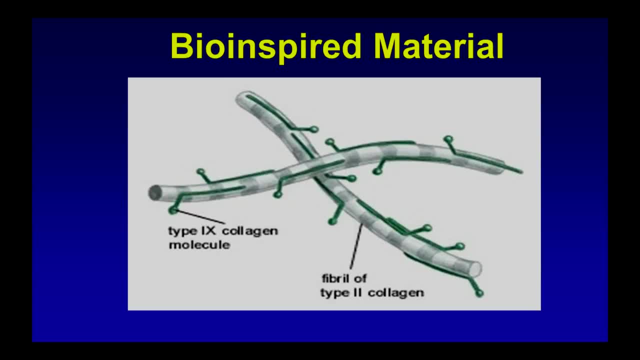 cells are actually seeing or sensing in the body, these kind of nano, very small features, And that's cueing them to turn it into this tissue. But we are looking very specifically at cartilage. Cartilage is made up of these very small fibers, collagen fibers. 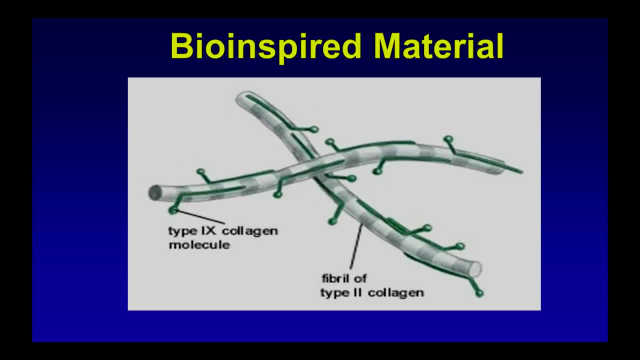 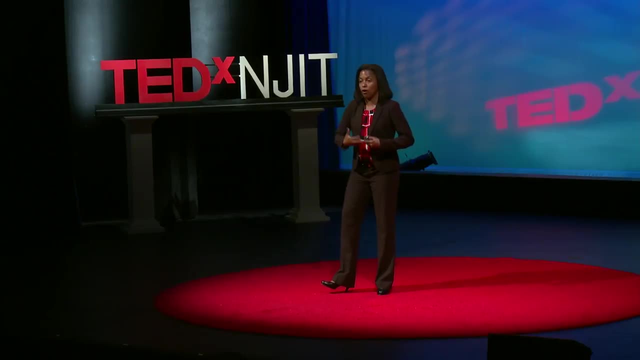 And these collagen fibers are decorated with a little more collagen, but also another specific type of molecule- It's called DAG, okay, or glycosaminoglycan, And what's interesting about this glycosaminoglycan is that actually helps to support all the mechanical loading that your knee undergoes. when you're walking, when you're running. It also helps to support biological activity. So it actually provides the cues to those cells because it actually combines with what we call growth factors And those factors stimulate, drive the cells to turn into these chondrocytes or cartilage cells. 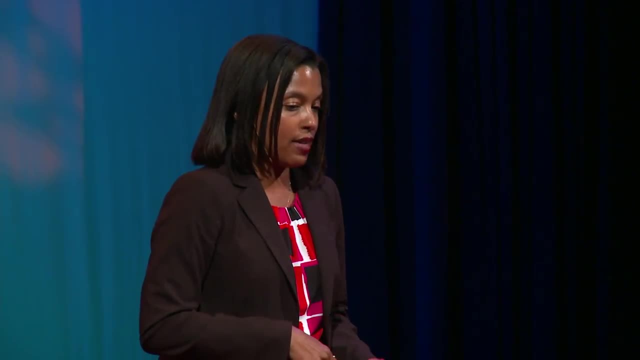 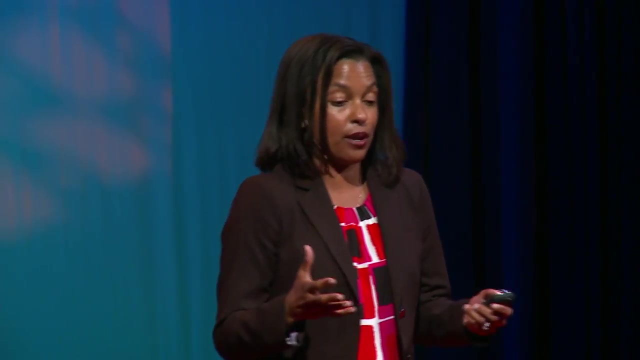 So we've been able to improve upon what's naturally there- that GAG- and created a GAG mimetic. Okay, so the chemistry is actually altered a little bit, so it becomes better, performs a little better, And what we've been able to show with the stem cells, with that GAG mimetic- 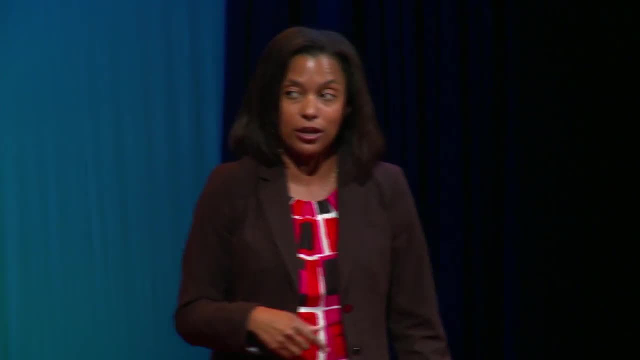 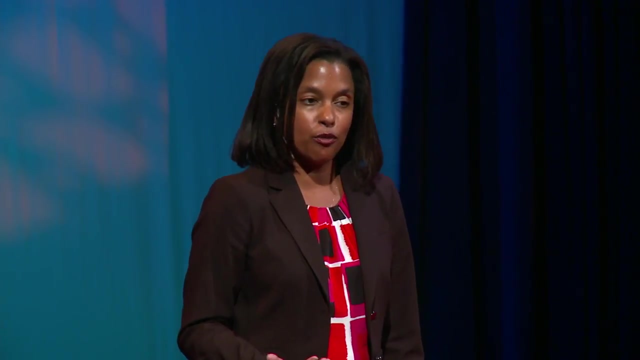 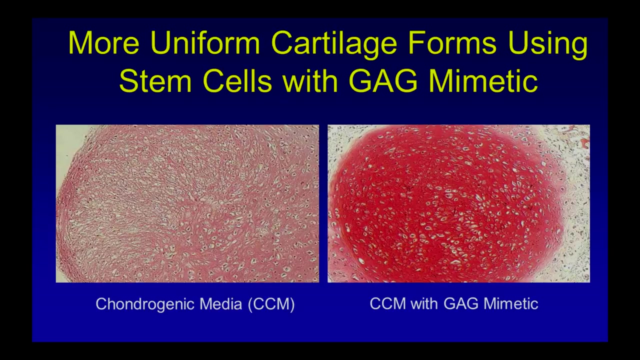 it actually drives them to turn into cartilage cells very quickly And they form a lot of cartilage tissue. So, shown there on the right, that intense pink stain is very uniform cartilage, articular cartilage tissue. So the cells look like cartilage cells and you've got a lot of that cartilage, a lot of cartilage tissue present. 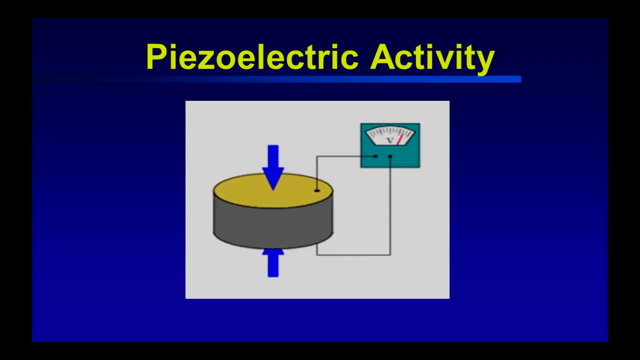 Another key interesting fact about those GAG materials is that it has another physical property called piezoelectric activity, And so what's important about that is, if you apply very small minute mechanical deformation, you'll get electrical stimulation. Okay, and so we then do make or create a bioinstrument. 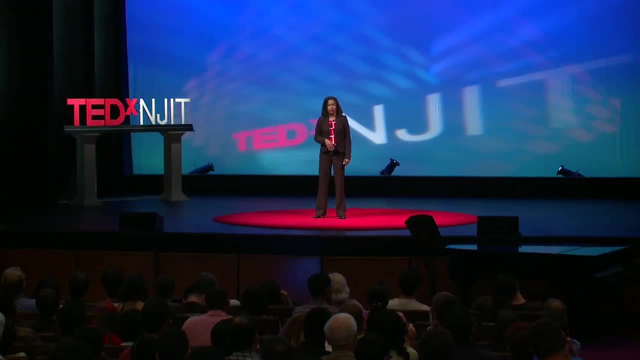 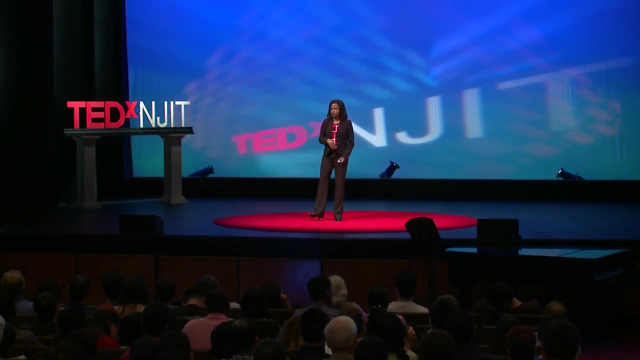 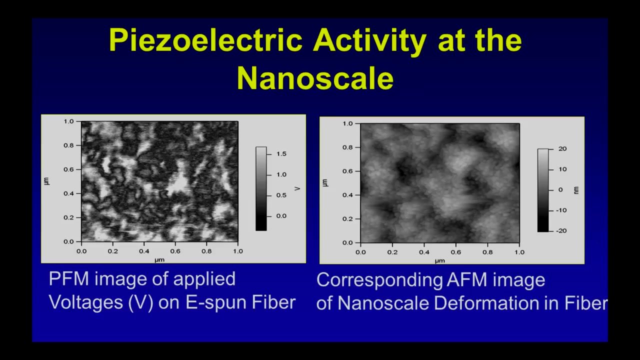 So we've created a piezoelectric material to actually get improved piezoelectric activity out of that material. So we apply a small little deformation and you get electrical stimulation And so this is happening at the nanoscale. So very small again. here is kind of reverse, is where you apply a voltage and you see this kind of deformation happening in the material at the nanoscale. 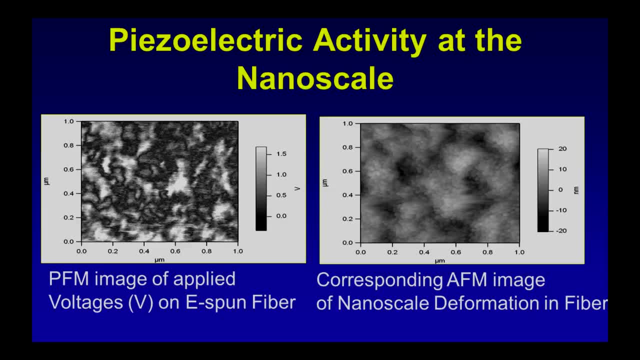 And that's important again for cueing the cells, Because they're attaching. They're attaching Their little feet are attaching to the materials at that nanoscale and it's stimulating them okay through this feature. So we've been able to show for cartilage again. it drives them to form cartilage. 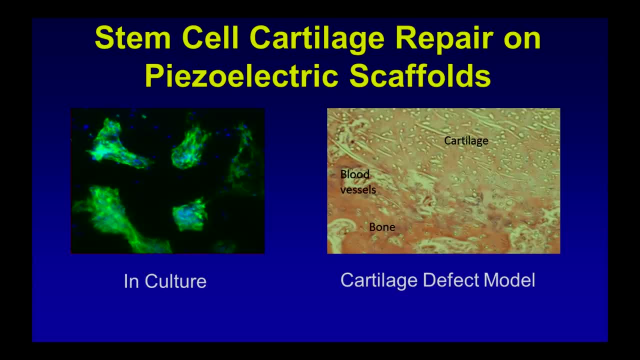 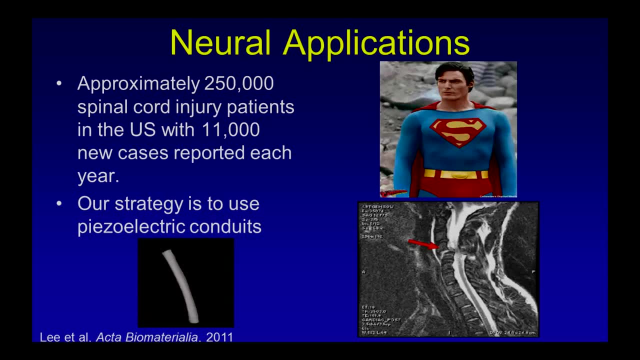 Okay, they form these aggregates and start to turn over and form cartilage tissue, And we've shown these in a defect as well- that they produce, make cartilage tissue. So I'm going to conclude here with the final, most challenging application, And this is something that we're dealing with in my laboratory. 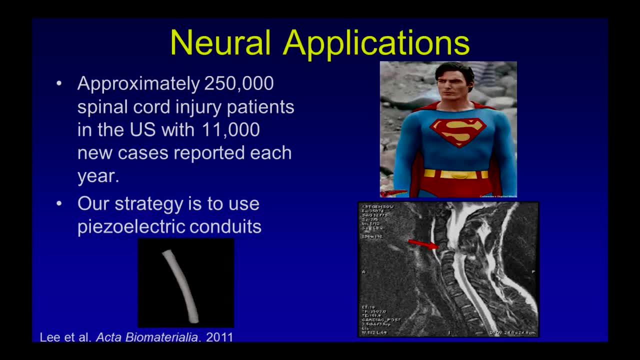 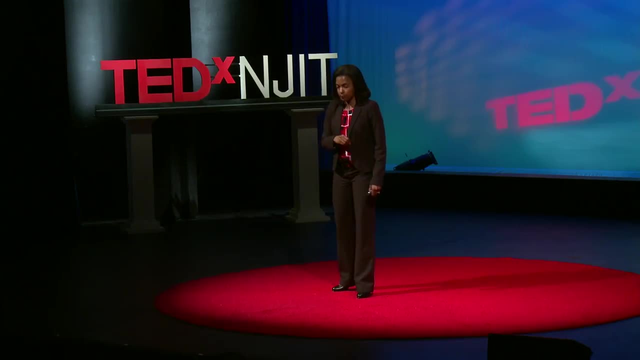 The area of neural spinal cord repair. And why is this so challenging? Okay, one of the most popular then people that have suffered from this injury is Superman, right? Or the actor Christopher Reeve, who played Superman. And, unfortunately, when you're injured to the spinal cord, okay, then this becomes completely devastating, debilitating. You can become completely paralyzed. okay, So there's over a quarter million people, then, suffering from this condition And that injury. unfortunately, the spinal cord does not have the ability to repair itself And there's currently, again, no treatment out there to actually repair it so that it's fully functioning. 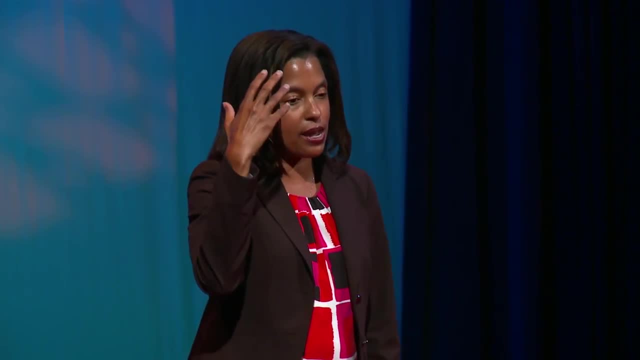 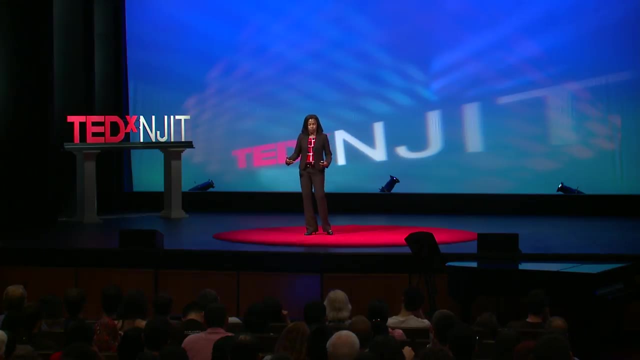 So the brain? essentially, once that injury occurs, the brain is then disconnected from the rest of your body. Signals from the brain travel down that spinal cord and connect you to the rest of your body, But that is no longer there, So we use what's called piezoelectric. 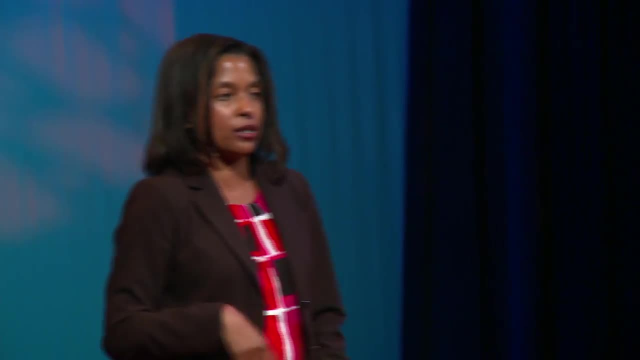 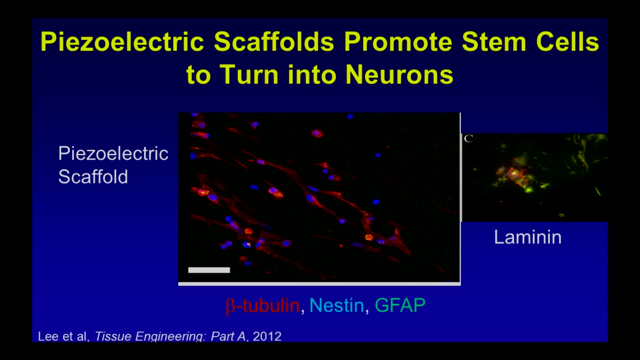 Conduits. okay, We're developing those piezoelectric materials that will stimulate the cord to actually regrow And we've been able to show with a different type of stem cell- we're using neural stem cells here- that if we put these on these materials they will drive them to become neurons and start extending these axons or these nerves. 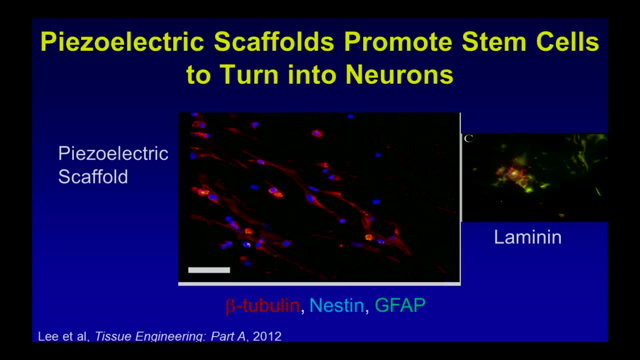 And shown here then are the red stain. These are the neurons that these stem cells have turned into. If you don't use that piezoelectric material you don't get those neurons to develop. So very interesting finding Again. the advantage here is this material has this intrinsic property. 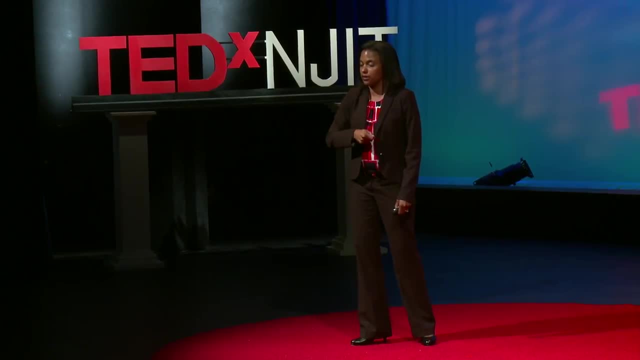 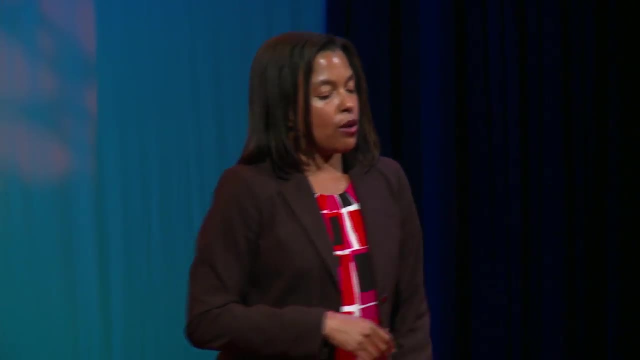 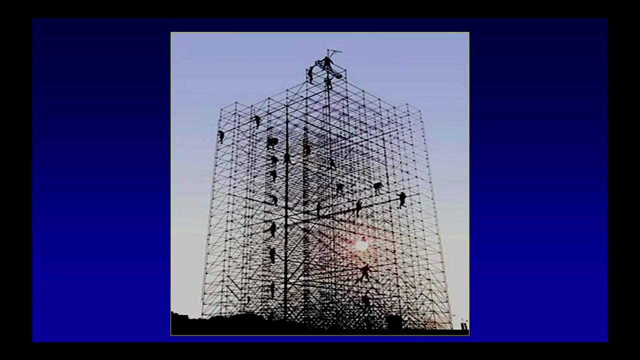 You don't have to use some external stimulation to get this to happen. The material itself will stimulate, cause electrical stimulation. So I just want to conclude here the importance of this technology and designing these scaffolds here to have these very small features, because they help the cells, support the cells and drive these cells to produce the tissue. 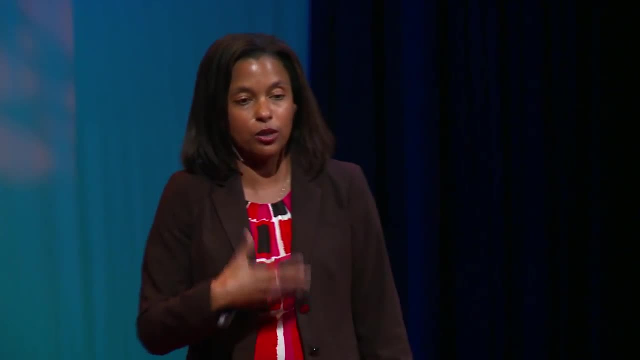 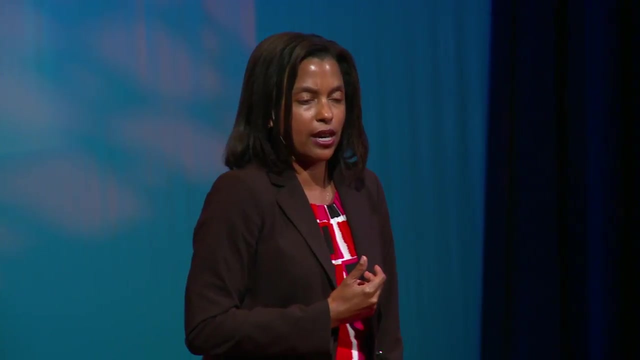 So we are developing this technology And our goal here, and really as a biomedical engineer, is to help these patients or improve the quality of life in these patients, So I would like to thank you.